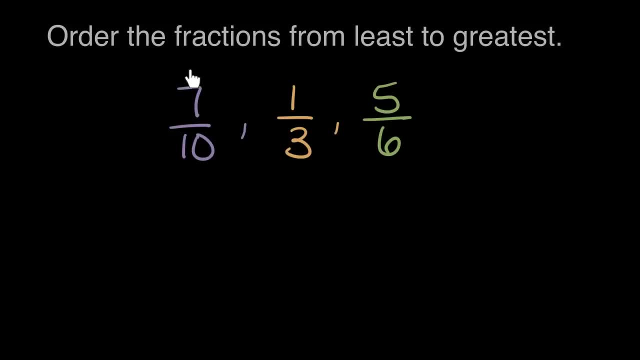 These two we could compare by estimating and see that this one, 7 tenths, is probably greater than 1 third. But then we get over here to 5 sixths and five out of six. well, again, that's most of the group. 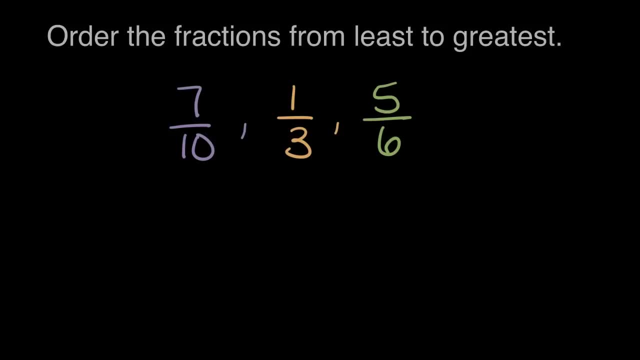 But is this most of the group- greater than the 7 tenths? most of the group? That gets a lot trickier. So what we can do is we can try to change these fractions to make them easier to compare So we don't have to compare tenths to thirds to sixths. 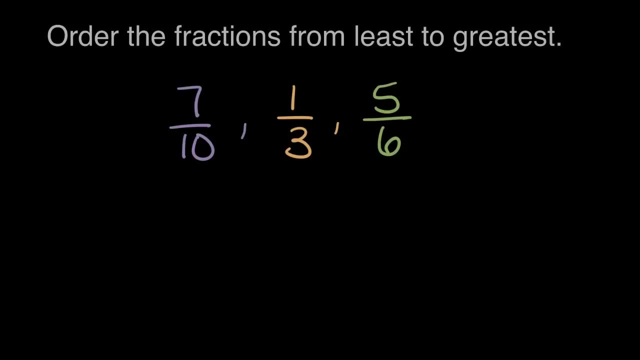 because those are all different sizes, different size groups, different size pieces. that's tricky to compare. So we wanna change these to be the same size. So we need some number, a multiple of 10,, 3, and 6, something we can multiply 10,, 3, and 6 by. 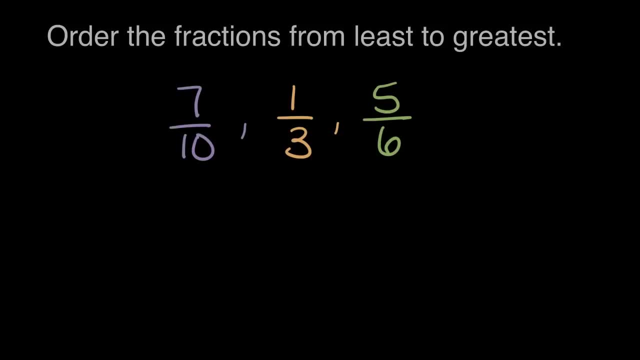 to get a new denominator that will work for all of the fractions. One way I like to figure this out is I look at the biggest denominator, which is 10, and I think of its multiples. The first multiple is 10, because 10 times 1 is 10.. 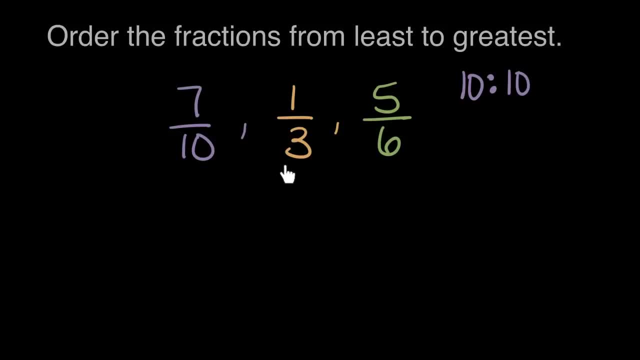 Can we change thirds and sixths to have 10 as a denominator? Is there any whole number? you can multiply 3 times to get 10? There's not, so we need to keep going. 10 doesn't work. The next multiple of 10 is 10 times 2,, which is 20.. 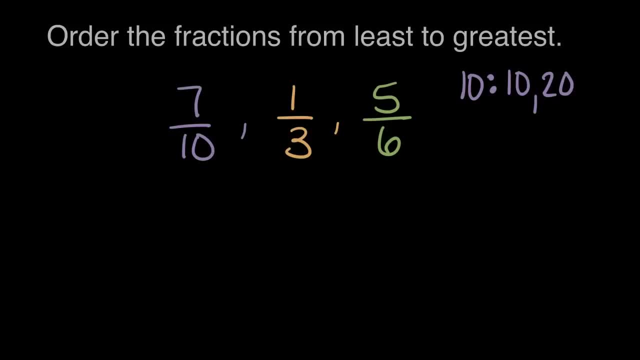 Again 3 and 6, is there a whole number? we can multiply them by to get 20? Again no. so 20 doesn't work. How about 30?? Let's see 3, we can multiply 3 times 10 to get 30,. 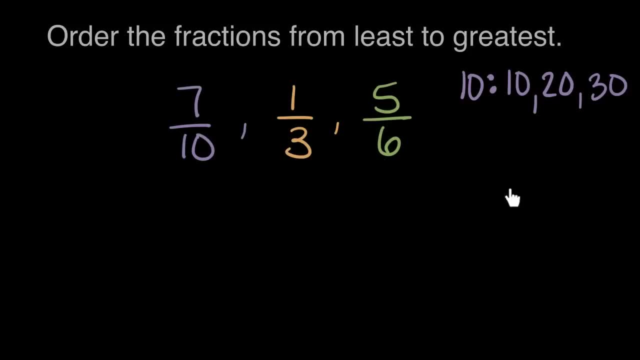 so 30 works for 3, how about 6?? 6 times 5 equals 10.. 6 times 5 equals 10.. 6 times 5 equals 10.. 6 times 5 equals 30, so yes, 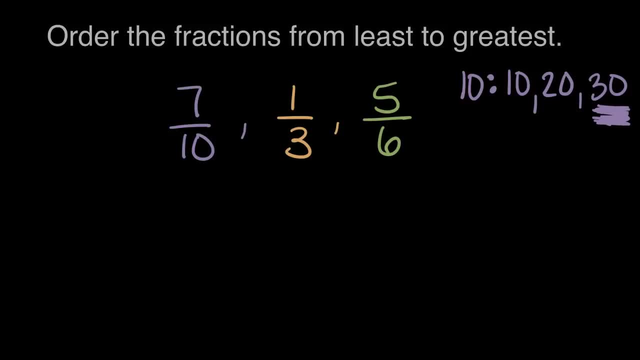 30 can work to be our common denominator. 30 is a multiple of 10,, 3, and 6.. So let's start converting our fractions to have denominators of 30.. We'll start with 7 tenths and we want it to have a denominator of 30.. 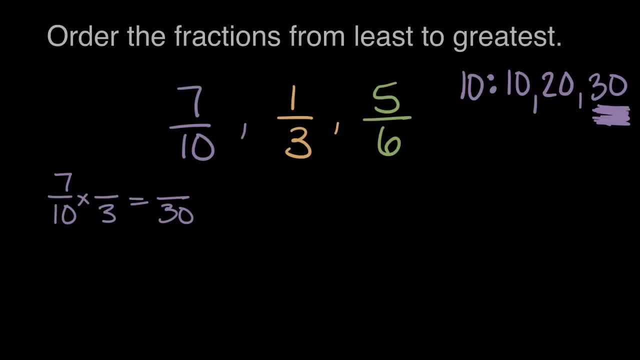 So what do we need to? multiply by 10 times 3 is 30. We always multiply the numerator and denominator by the same number. So 7 times 3 is 21.. So 7 tenths is equal to 21 thirtieths. 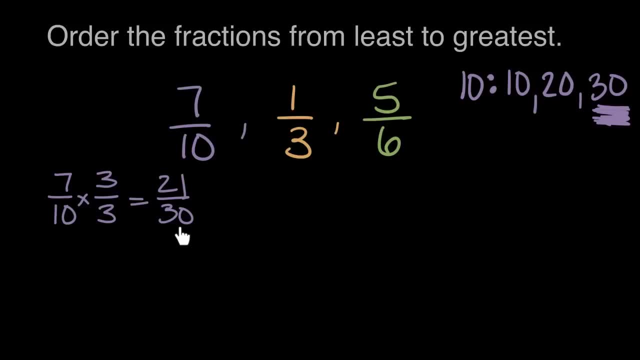 These are equal. we've just changed the size of the group. We've changed the denominator so that they will be easier to compare, but we've not changed what portion of the group we're representing. 7 out of 10 is the same portion as 21 out of 30.. 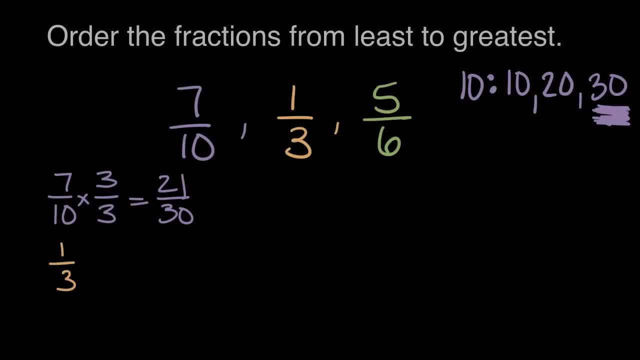 And then let's keep going with 1. third: Again, we want a denominator of 30, so this time we'll multiply 3 times 10 to get 30. Again, numerator also times 10.. 1 times 10 is 10.. 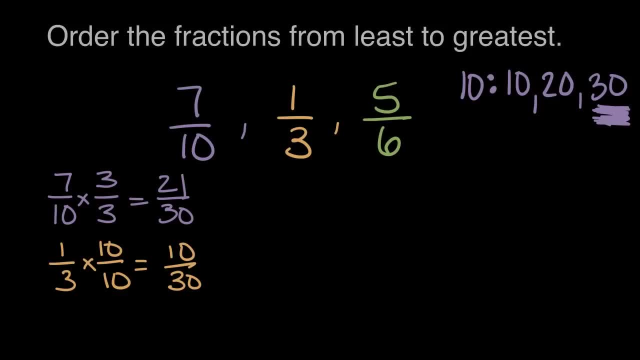 10 out of 30 is the same as 1 third. If you have 10 of the 30 people again, we'll use the wear glasses example- or 1 third. that is the same size of the group, the same portion. 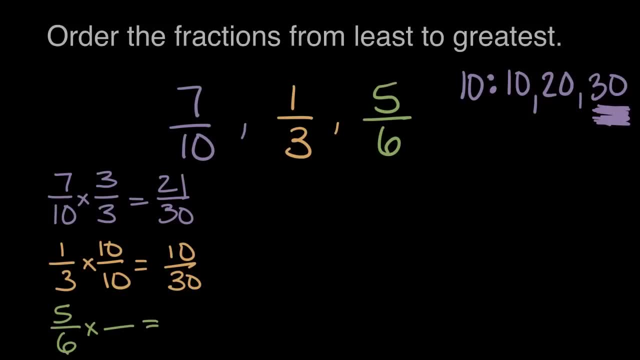 And finally, 5 sixths. what do we need to multiply here to get 30?? 6 times 5 is 30. So we multiply the numerator times 5, and 5 times 5 is 25.. So now, instead of these original fractions, 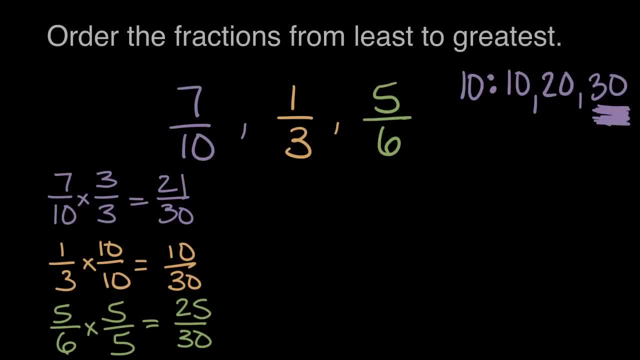 that were tricky to compare. we have much easier numbers to compare. We have 21 thirtieths, 10 thirtieths and 25 thirtieths and 25 thirtieths. In this case, the pieces are all thirtieths. 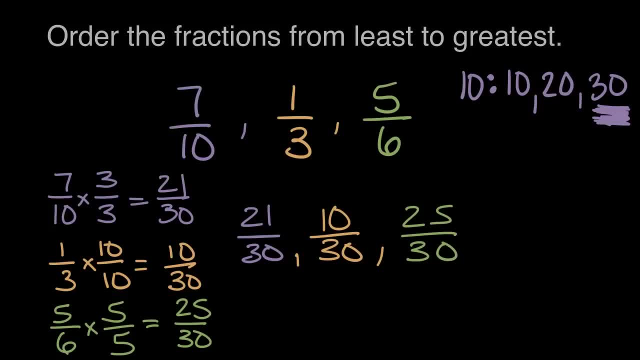 They're all groups of 30, so this is much easier to compare. We can simply look at the numerators to see what portion of those 30 the fraction represents. So the first 7 tenths is the same as 21 out of 30,. 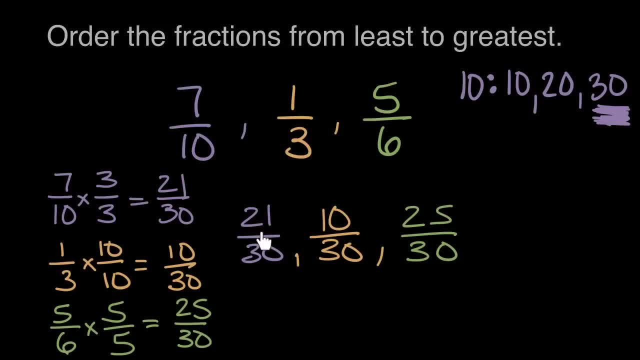 whereas 1 third is 10 out of 30. Well, clearly 21 out of 30 is a larger portion of the group than 10 out of 30. So we were right. We estimated up here that 7 tenths is larger than 1 third. 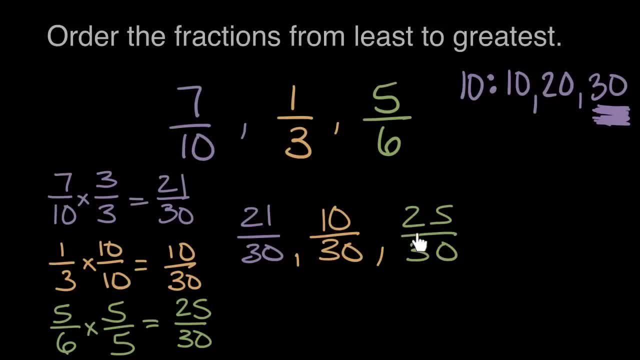 But then the trickier one over here. now we can see much more clearly: 25 out of 30 is the greatest portion of the group. 25 is more than the 10 or the 21.. So we can list these now from least to greatest. 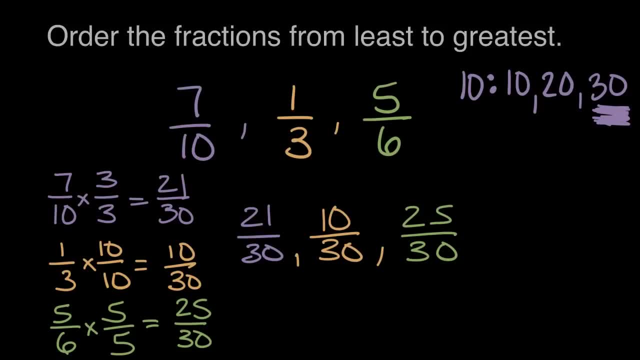 The least. the smallest is 10 thirtieths, which again remember, is equal to 1 third. So we can put: 1 third is least and we can cross that off. Next it's either 21 out of 30 or 25.. 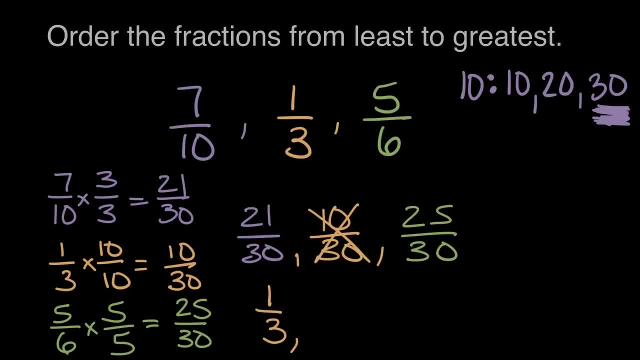 21 is less and that represented 7 tenths. So we can say 7 tenths, because 21 thirtieths equals 7 tenths, And finally that leaves us with 25 thirtieths. 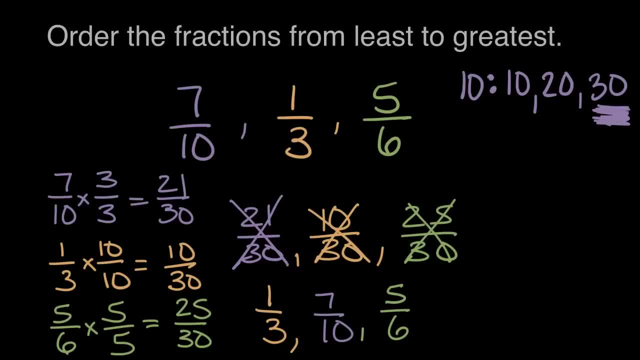 which is equivalent to 5 sixths. So, from least to greatest, our fractions are 1, third, 7 tenths and then 5 sixths. 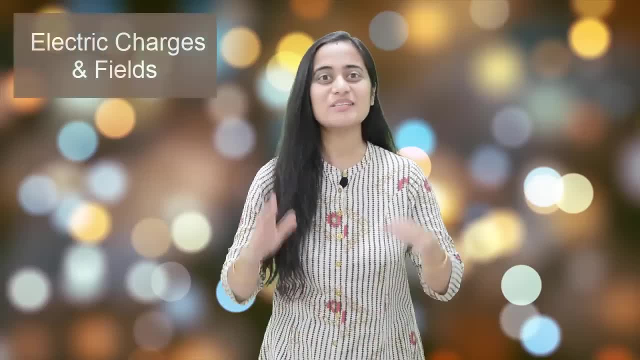 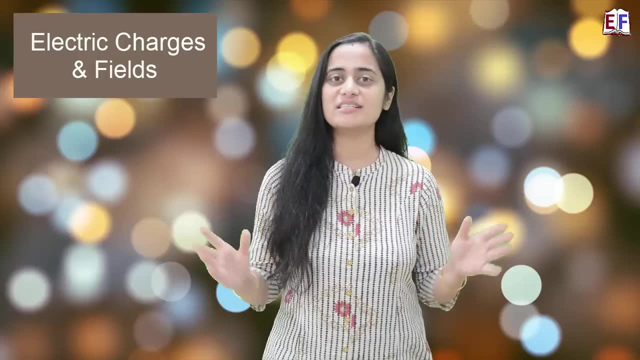 Hello everyone, I hope all of you are doing good and today we are going to learn about electric charges and fields in one video. Yes, so this is a crash course video on electric charges and fields and we are going to cover all the theory, all the concepts and few numericals. 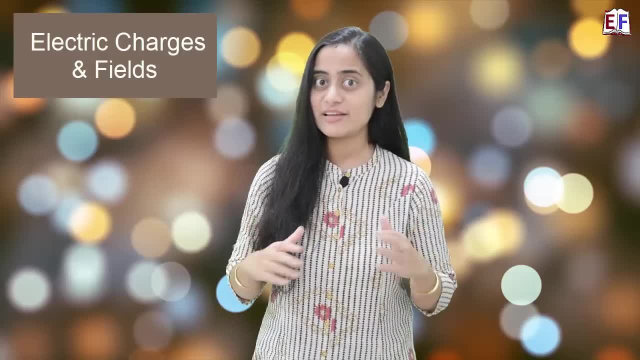 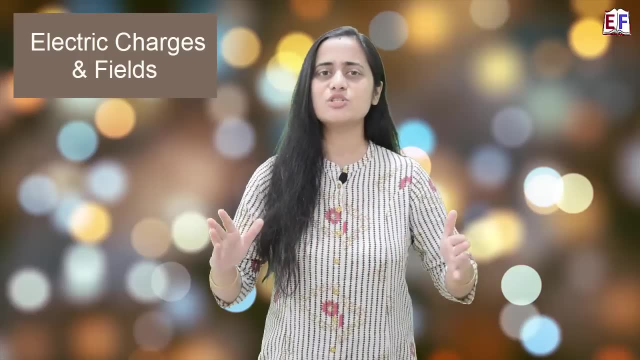 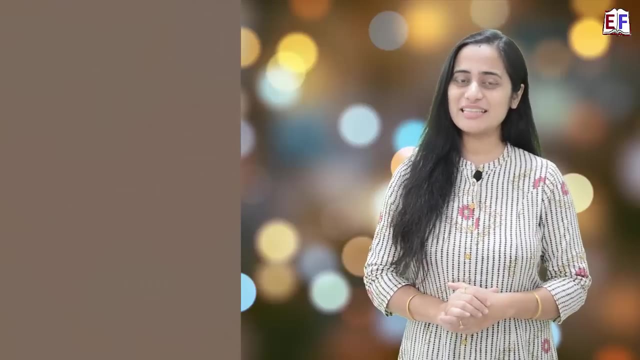 as well. However, if you are looking for detailed derivations and more numericals, please refer to the link which is given in the description section. We have made detailed videos on electric charges and fields. Some of the topics that we are going to cover in this video are Coulomb's law.